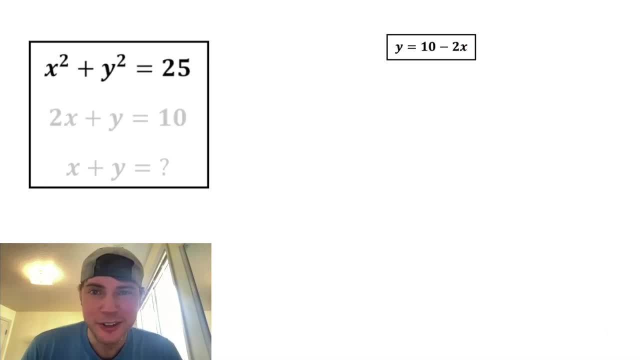 Next, let's focus on the x squared plus y squared equals 25.. Let's bring it down and in the place of this y right here, I want to plug in 10 minus 2x. So now this is 10 minus 2x being squared. so we're going to multiply 10 minus 2x times 10 minus 2x. 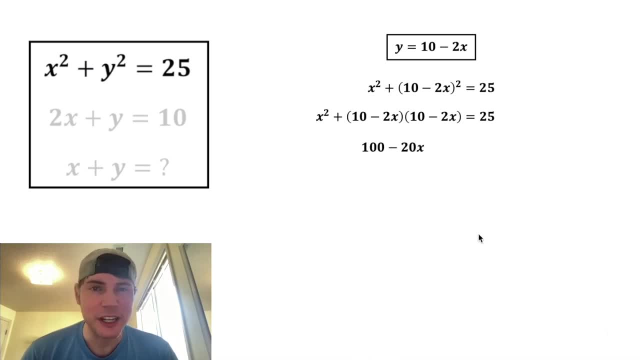 10 times 10 is 100.. 10 times negative 2x is negative 20x. Negative 2x times 10 is negative 20x and negative 2x times negative 2x is positive 4x squared. 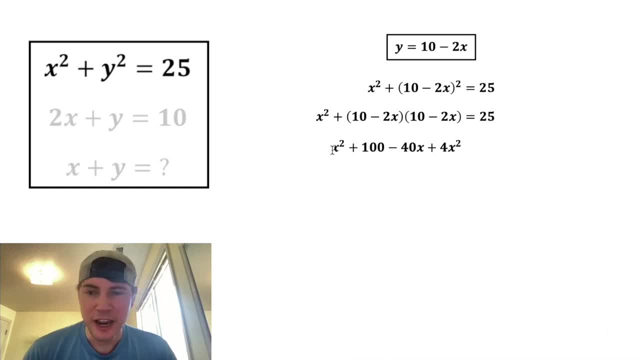 And these two can combine to become negative 40x. Let's bring down the x squared and bring down the equals 25.. Anytime I do one of these several people always mention: why don't I do this shortcut? Well, I did try it out and it ended up not being much of a shortcut. 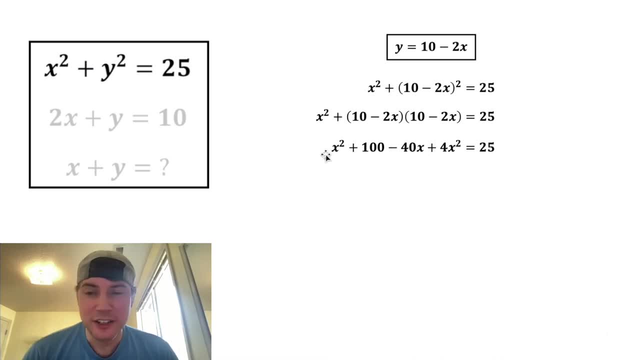 It doesn't flow as nicely as this method in these videos. So now let's combine like terms: x squared plus 4x squared is 5x squared, We can bring down the negative 40x, And if we subtract 25 from both sides, 100 minus 25 is 75, and 25 minus 25 is 0.. 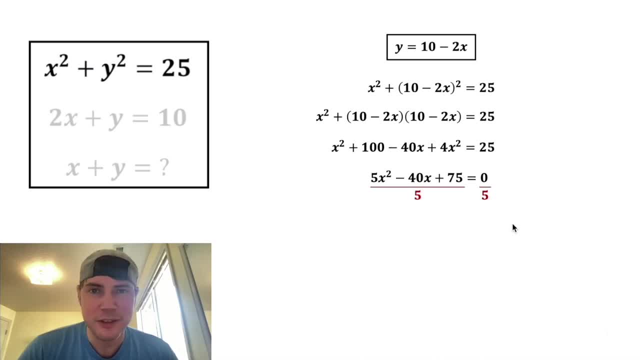 From here, all three of these terms are divisible by 5, so let's divide both sides by 5.. Each of these terms will divide by 5 to give us x squared minus 8x plus 15, and it's still equal to 0.. 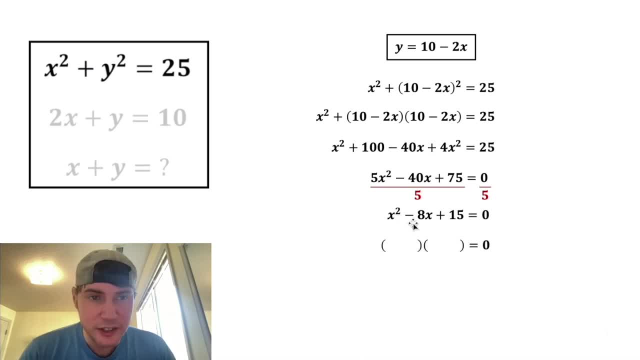 And now to solve this, we want a factor, We want two numbers that will add to negative 8.. And multiply to positive 15.. Well, negative 3 plus negative 5 will give us negative 8. And negative 3 times negative 5 will give us positive 15.. 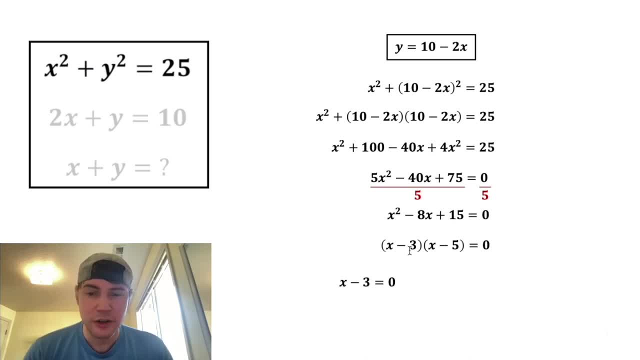 So these are the factors of this. So from here, if this equals 0, or if this equals 0,, the whole thing will equal 0. Because anything times 0 equals 0. So we have this or this, And if we add 3 to both sides, we get x equals 3.. 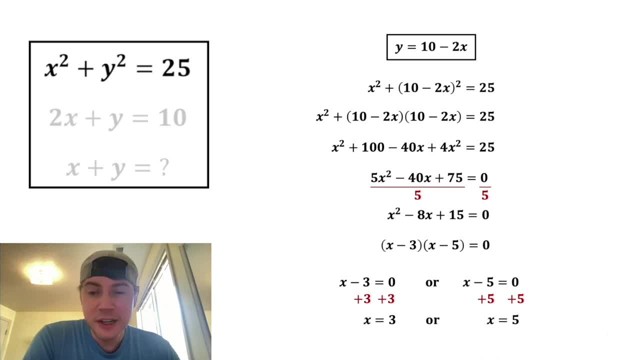 And if we add 5 to both sides, we get x equals 5.. So x can be either 3 or 5.. So we don't really need any of this work anymore and let's bring these up here. Since our goal is to figure out what is x plus y, we want to find out our corresponding y values. 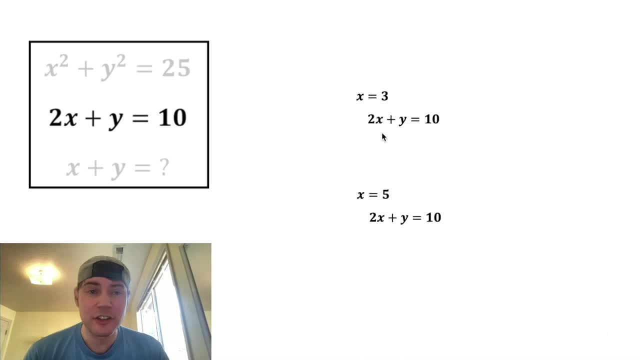 So let's use this: 2x plus y equals 10.. We'll copy it down. solve for y in the place of this x. Let's plug in 3.. 2 times 3 is 6.. Let's subtract 6 from both sides and we get y equals 4.. 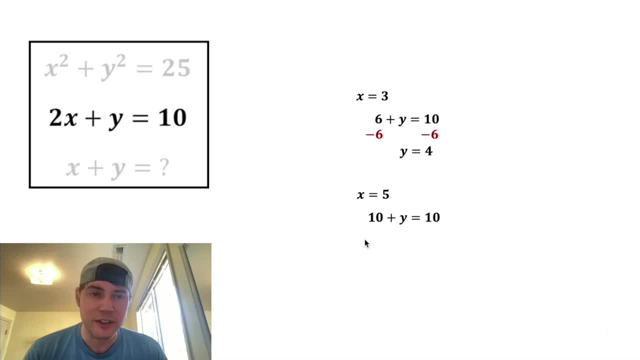 And same thing for this one. If we plug in 5 for the x, 2 times 5 is 10.. Subtract 10 from both sides and we get y equals 0. These are our two possible scenarios And we want to evaluate x plus y for each of these scenarios.